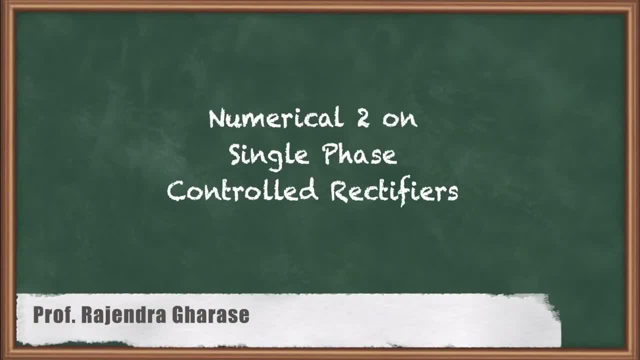 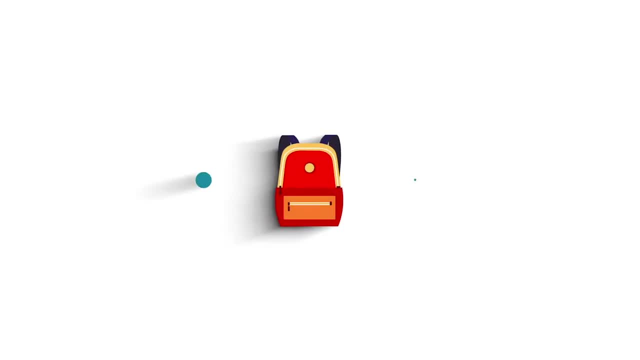 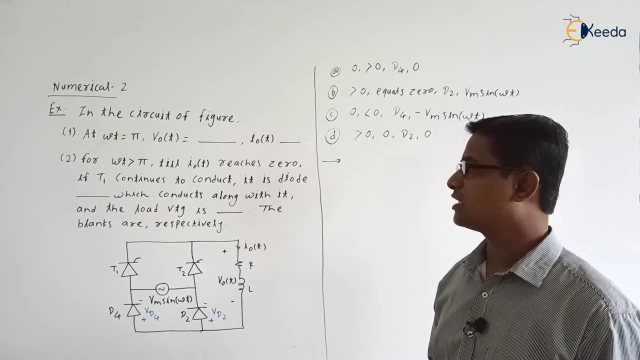 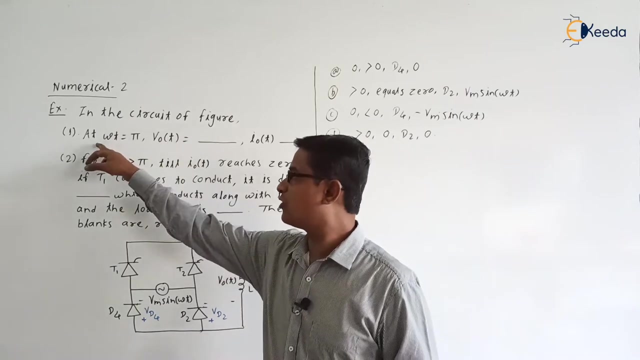 Hello friends, now we are going to discuss the second numerical, that is the numerical 2.. Let us read the numerical carefully. In the circuit of figure at omega, t is equal to pi. V0 of t is blank space they have given. 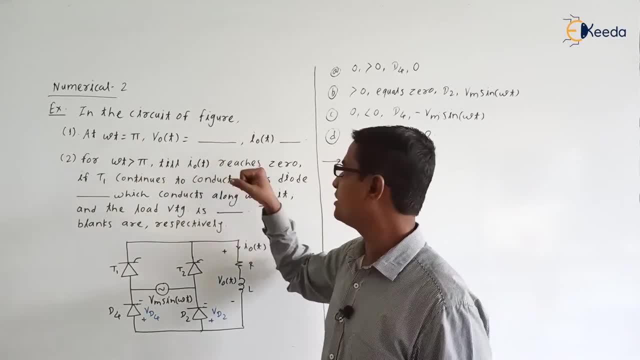 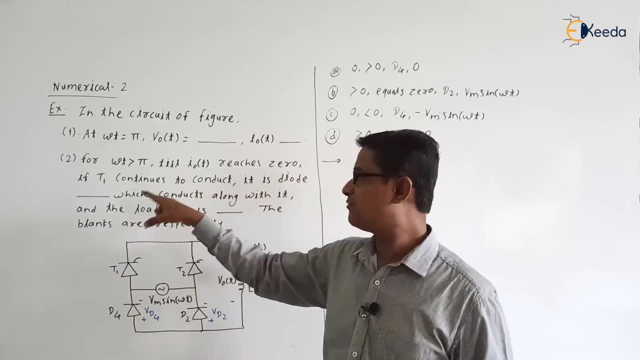 Means it is expected that what is the value of V0 of t right, I0 of t blank space? second for omega, t greater than pi till I0 of t reaches 0. If t1 continues to conduct, it is diode blank space which conducts along with it. 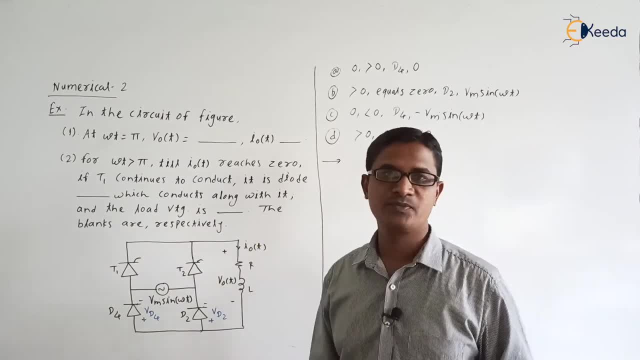 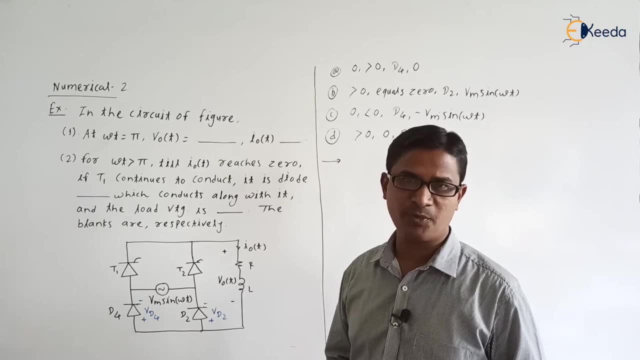 And the load voltage is blank space. the blanks are respectively okay And they have given. yes, it is a symmetrical configuration and the half controlled bridge rectifier. Are you getting the point? Okay? One thyristor, one diode. one thyristor, one diode. 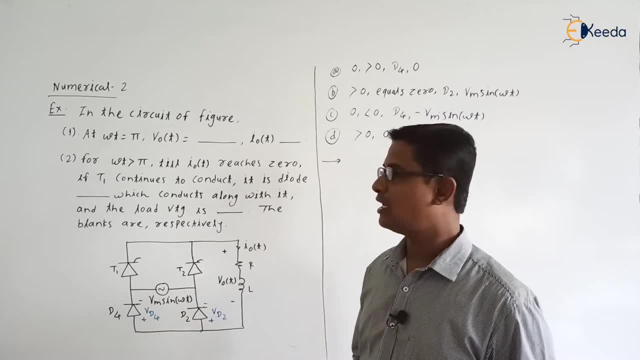 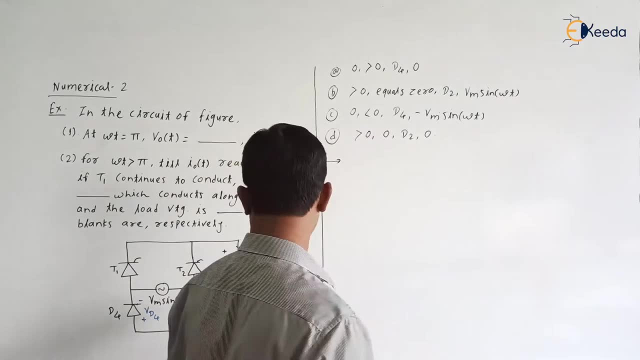 Okay, Vs is Vm into sin of omega t. right Now, they have asked the specifically questions regarding V0 of t, I0 of t and which diode conducts. okay, So for this circuit can we draw the waveform? Yes, we have already discussed about this circuit. 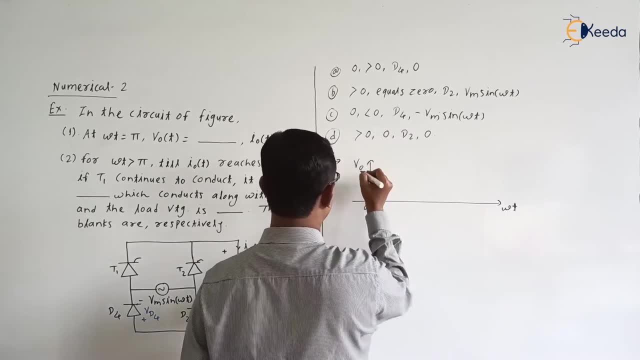 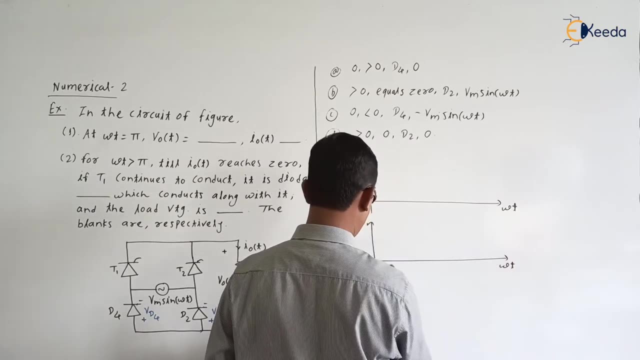 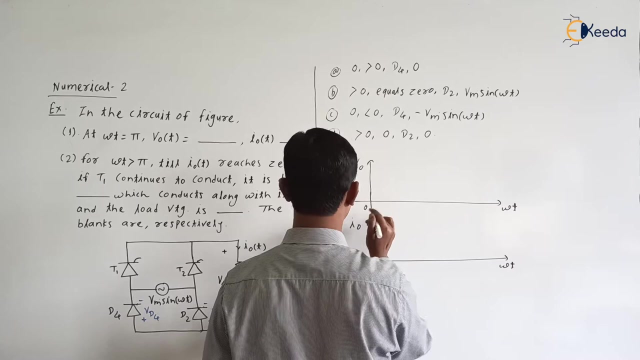 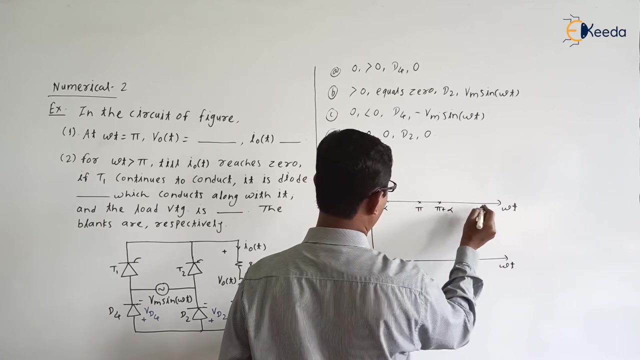 Zero. this is omega t Suppose, this is V0 and next let us draw the I0 as well. Omega t load: they have given it as a RL right Load, they have given it as a RL Right. So if you check from, omega t is equal to 0 to alpha, alpha to pi, pi to pi plus alpha and pi plus alpha to 2pi. okay, 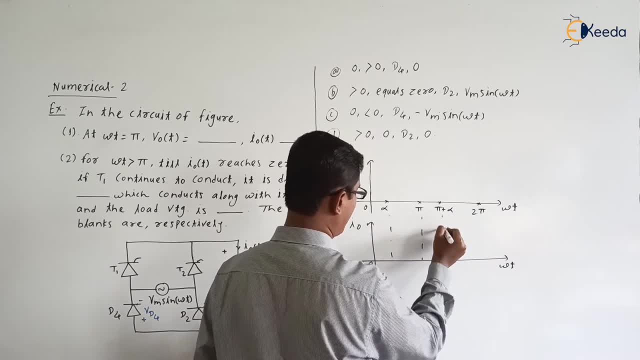 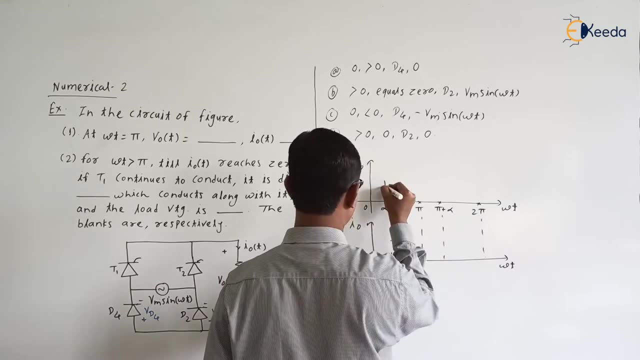 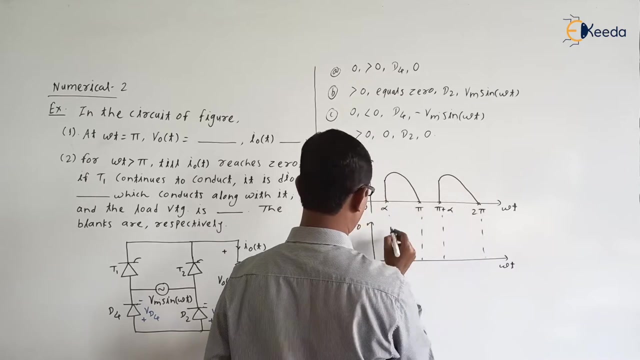 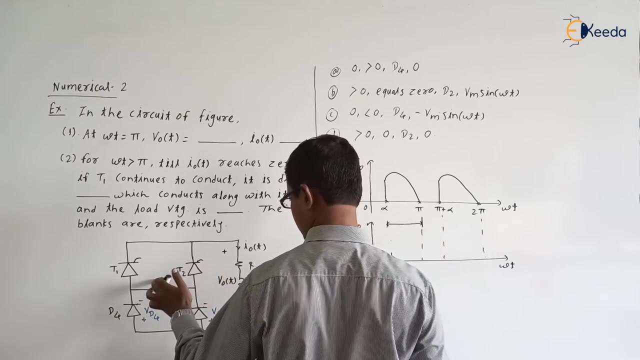 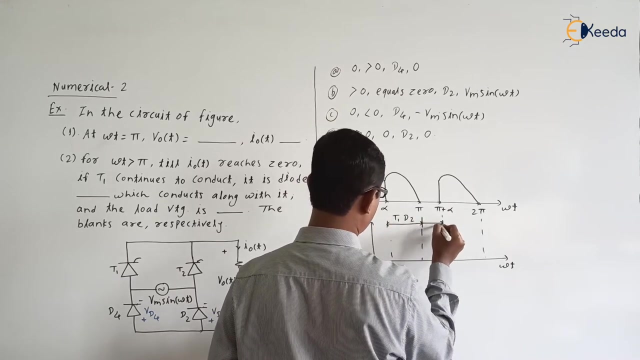 So alpha, pi, pi plus alpha, 2pi, okay. So here the output voltage will be like this: okay, During alpha to pi: yes, thyristor, T1 and D2, right Conducts. so here T1, D2 and from pi to pi plus alpha. whatever the energy stored by the inductor, inductor releases the energy through D4, T1. 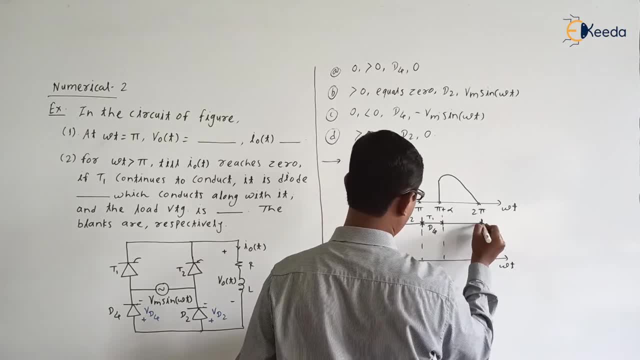 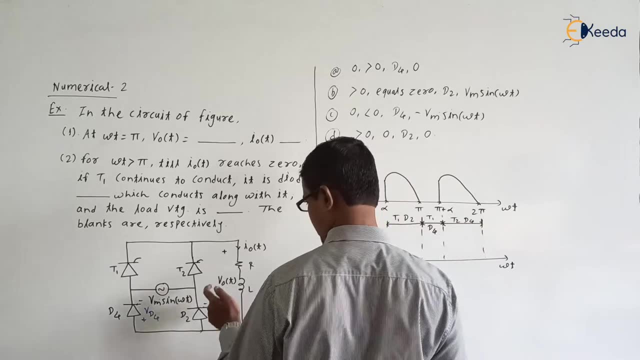 T1, D4. After that, pi plus alpha to 2pi, If you check it is T2, D4.. T2, D4. And here with T2, D2 will be in the conduction mode. okay. 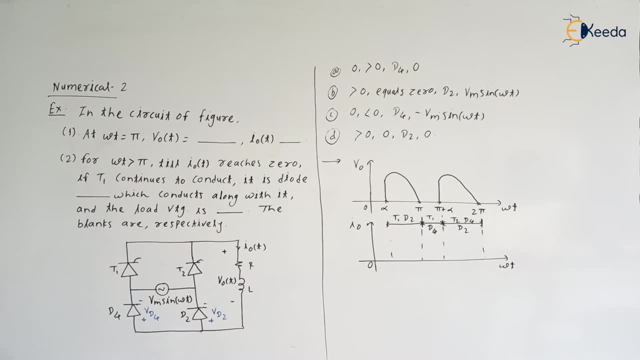 So if you check, yes for this circuit right, Vm sine omega t. So here it is a plus, here it is a minus during the positive half cycle. okay, So if you check at alpha thyristor T1 will be turned on. 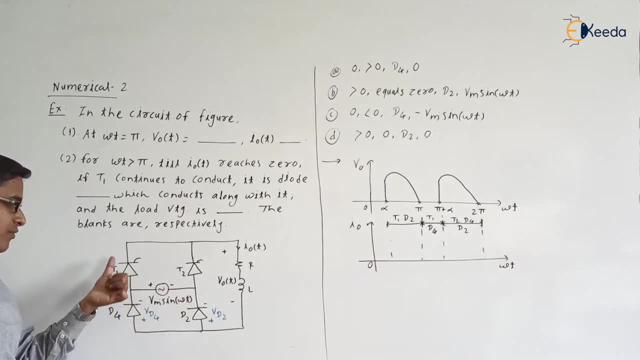 So current will be flowing from T1, load D2 and again back to the Vs. In this loop the current will be flowing right. So, inductor, go on storing the energy right. Inductor, go on storing the energy right. 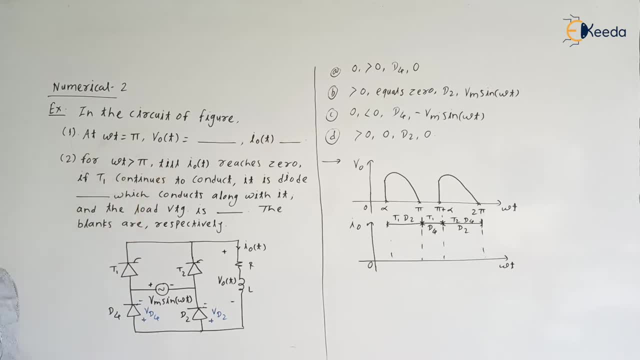 So if you check at, omega t is equal to pi, V0 of t is equal to. if you check at omega t is equal to pi, What is V0?? It is a 0, okay, So here V0 should be equal to 0, right. 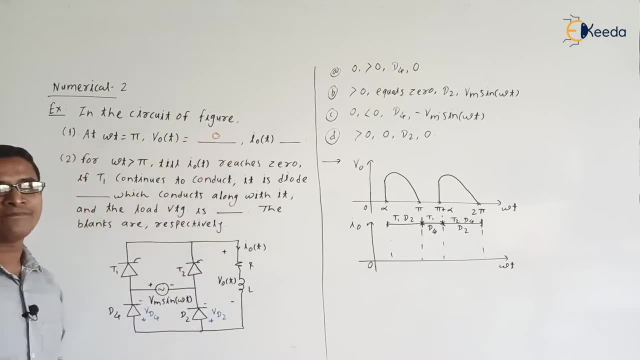 V0 is equal to 0. Is this clear? I0 of t. I0 of t. we need to find okay. So here, if you check, if the inductor is high, whether they have specified anything regarding the inductor. no, okay. 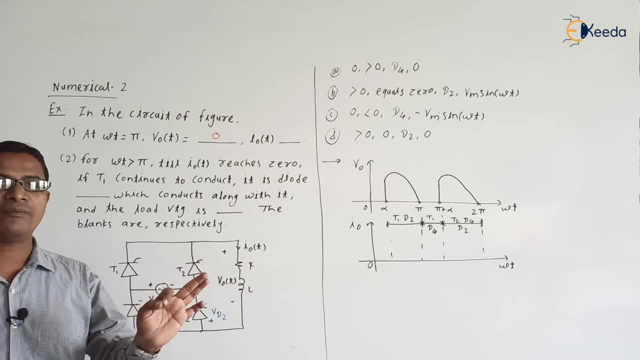 So let us consider, the inductor is having a lesser value. okay, So due to that, the conduction will be discontinued. Yes, okay, Because they have used the word for omega t greater than pi till I0 of t reaches 0.. 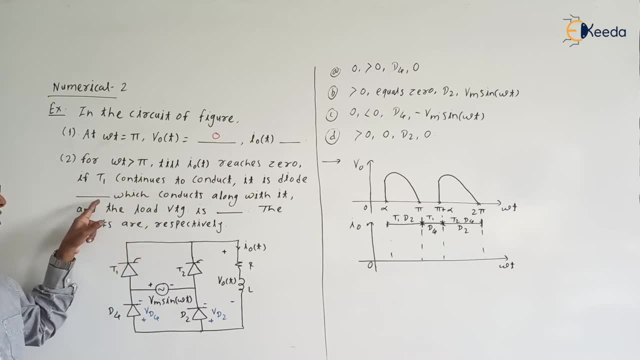 If T1 continues to conduct, it is diode dash dash which conducts along with it. okay, So till I0 of t reaches 0, they have said: okay, I0 is reaching the 0 means what It is: a discontinuous conduction, okay. 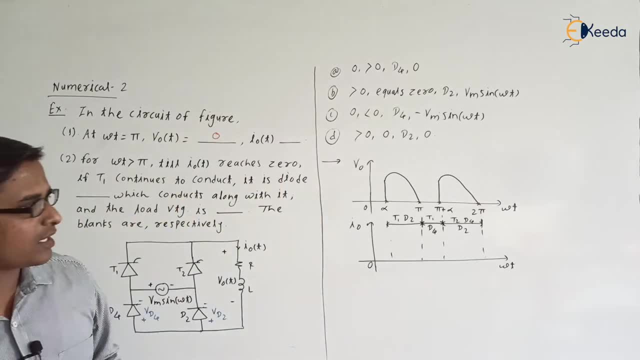 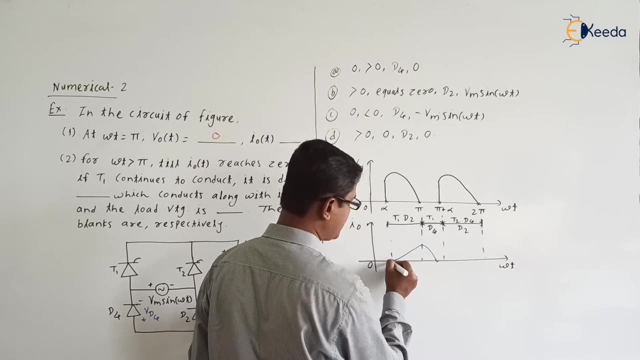 So after alpha, what is happening? After alpha, the inductor go on storing the energy. So from alpha to pi, inductor stores the energy right, And from pi to beta- suppose this is the inductor We are having. okay, 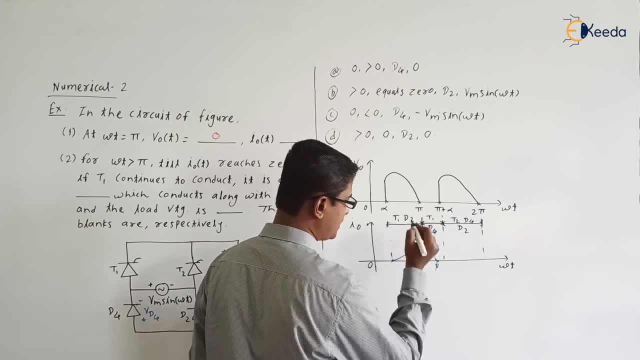 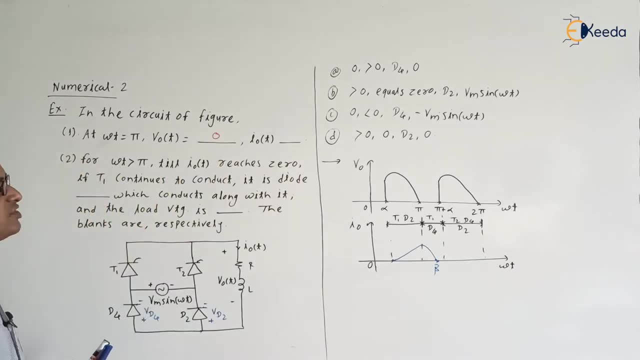 Lesser value of inductor. okay, So that's why it is reaching 0 means it is a beta, right? Suppose it is reaching 0 at beta. okay, So next. so what is the I0 of t? If you check I0 of t at omega, t is equal to pi. 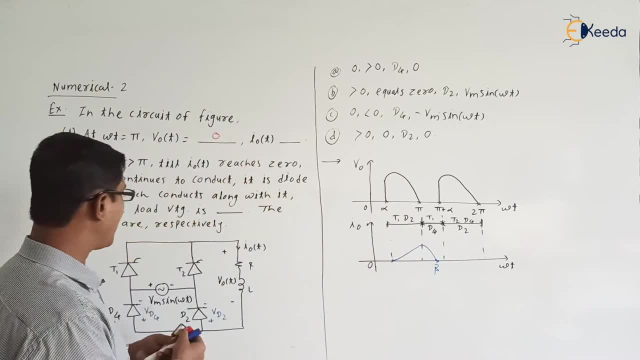 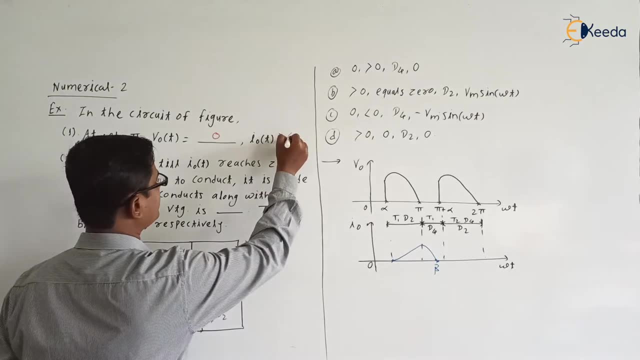 At pi I0 of t is positive, only okay. So at pi I0 of t is a positive. Positive means what It is: a greater than 0,. it is a greater than 0, right. I0 of t is greater than 0, right. 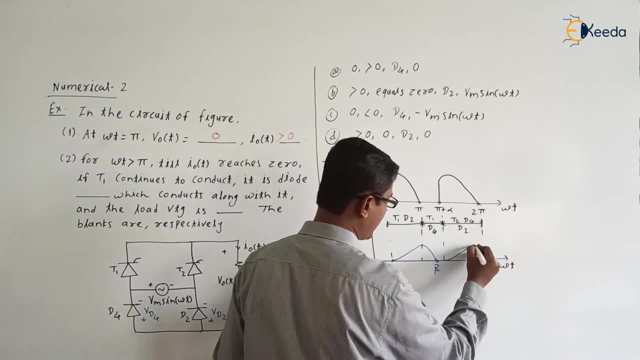 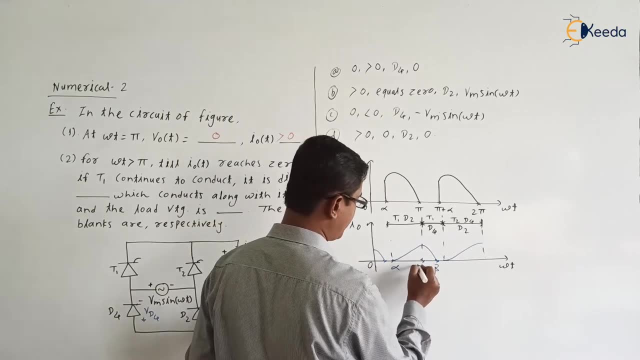 Next again. After that, what will happen At pi plus alpha? again, inductor stores the energy, and here it will be decreasing for the continuous cycle. okay, So it is a alpha, here it is a pi, beta, pi plus alpha, and here it is a 2pi- okay. 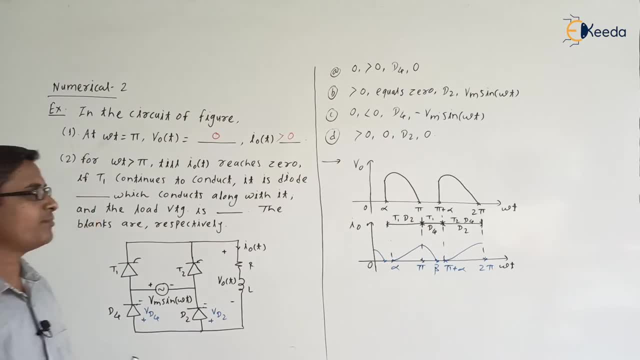 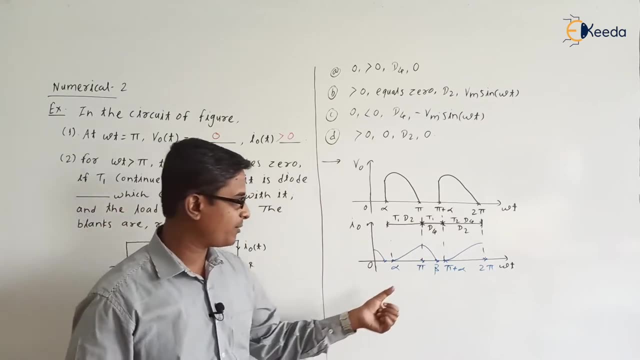 So next for the second statement. for omega t greater than pi means for omega t greater than pi means after this pi: okay, Till I0 of t reaches 0, means till after this instant, till I0 of t reaches 0, that is a beta okay. 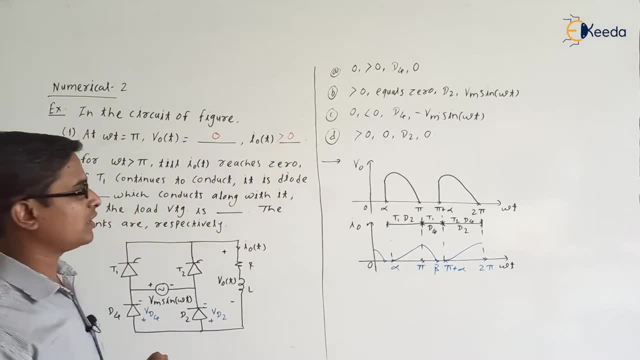 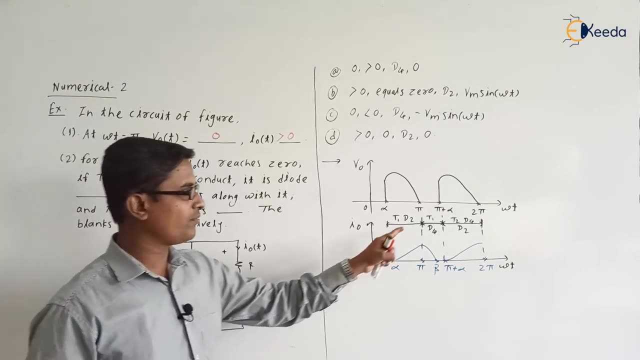 That is a beta. Yes, if t1 continues to conduct. if t1 is continuous to conduct, then it is the diode which conducts along with it. Yes, if you check with a t1, diode d4 will be in the conduction mode, okay. 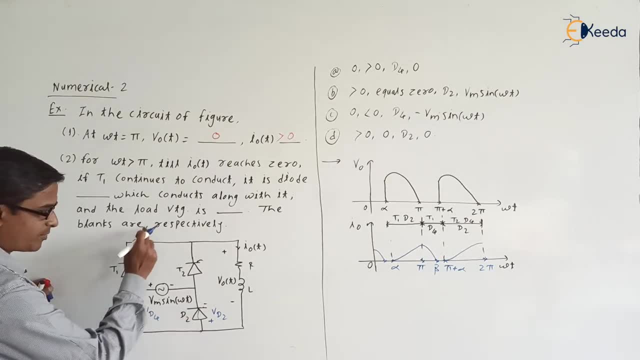 So here, when t1, d2 on state current flows from supply voltage t1, load d2 and again back to the supply voltage, inductor stores the energy, okay, After pi, what will happen? Supply voltage polarity is reversed. that means plus here and here it is a minus. okay. 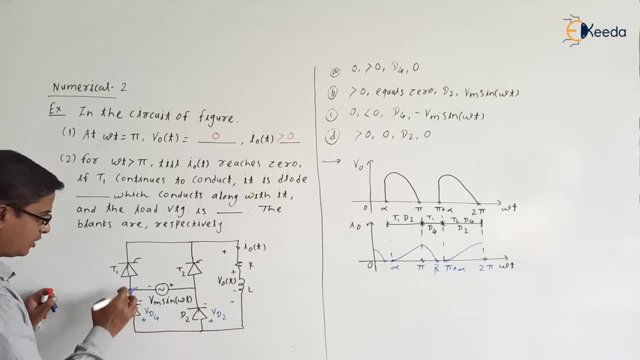 So here the inductor releases the energy. Okay, So here the inductor releases the energy Through d4, t1, through d4, t1.. So with t1, diode d4 will be there, okay. 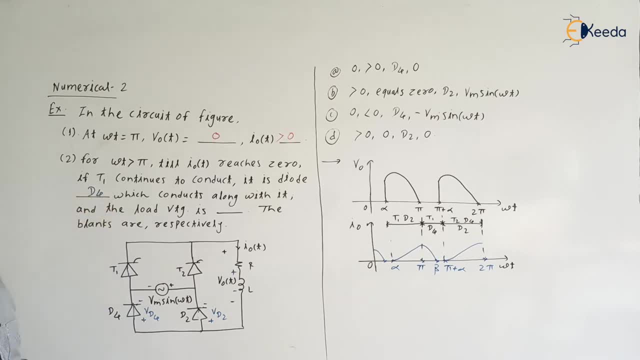 Diode d4, right, which conducts along with it. Is this clear? And the load voltage is, if you check during this interval means when these two are in the on state. what is the load voltage? Load voltage will be yes. voltage across the conducting switches is equal to 0. 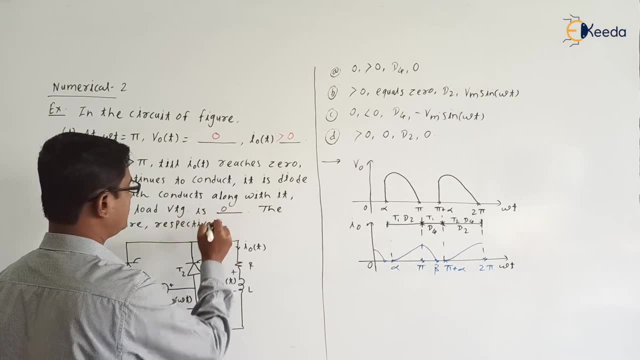 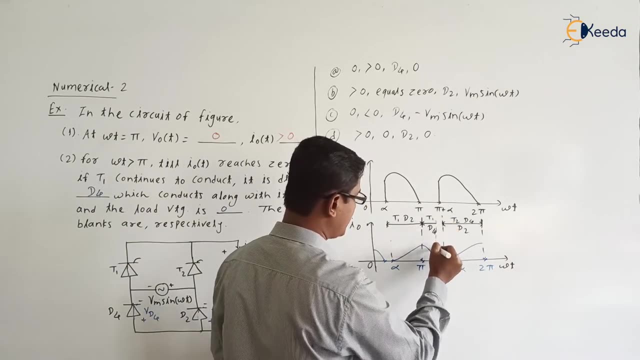 Yes or no, right? So load voltage is 0.. Is this clear? So please try to understand the circuit operation. This is a discontinuous conduction. This is a discontinuous conduction. So, due to that, what is happening? 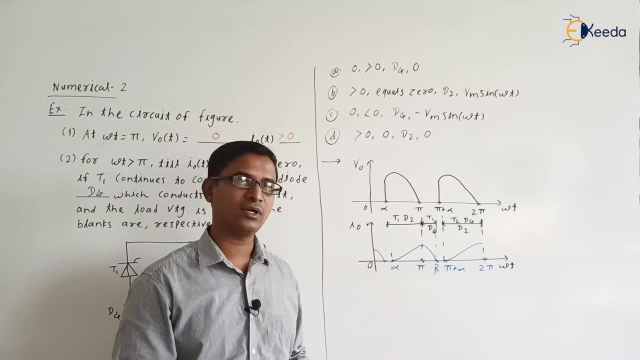 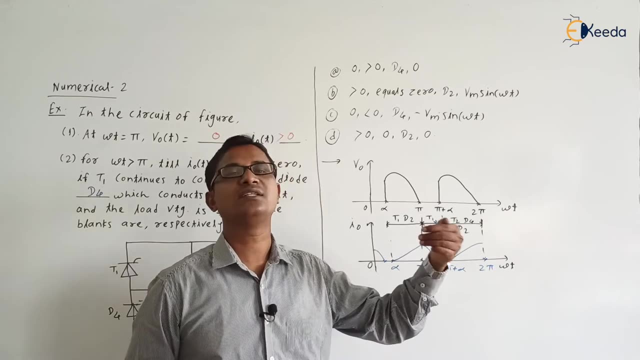 Yes, inductor is releasing the energy through t1, d4, right. But before applying the gate signal to thyristor t2, right. inductor releases the energy and whatever the induct, the inductor energy becomes 0, right. 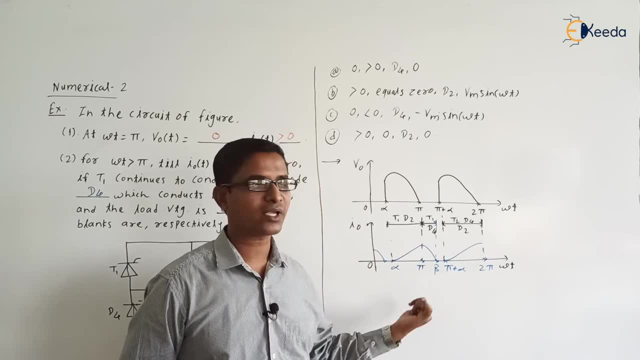 Before this instant inductor energy becomes 0,. that is at beta, okay. So here, if you check, yes, 0 greater than 0, d4 and 0,. 0 greater than 0, d4 and 0.. 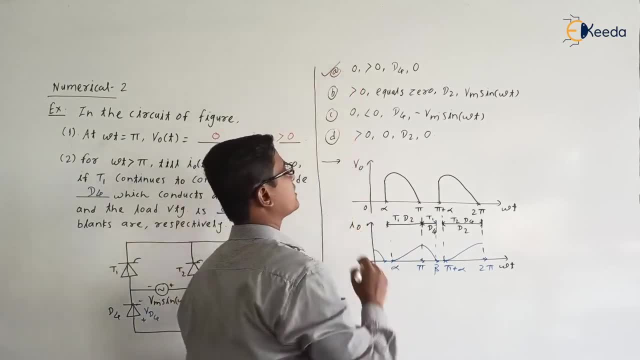 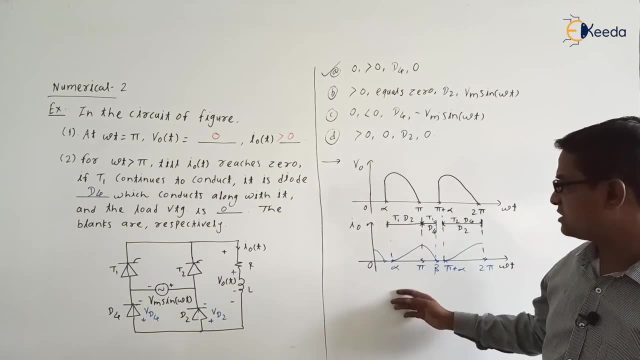 So correct answer is option A. Option A is the correct answer. Is this clear? Are you getting the point? Okay? so this is about the numerical two. Please try to understand. This is the discontinuous conduction. Okay means the value of the induct is lesser.